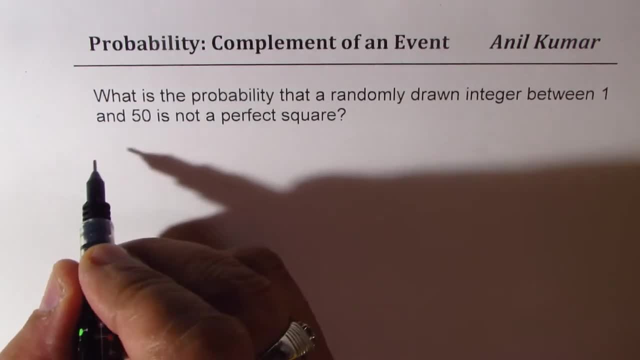 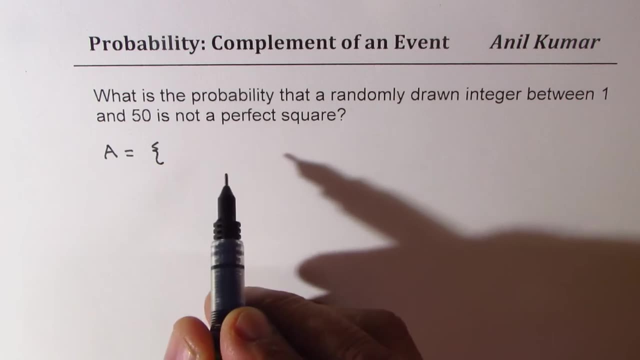 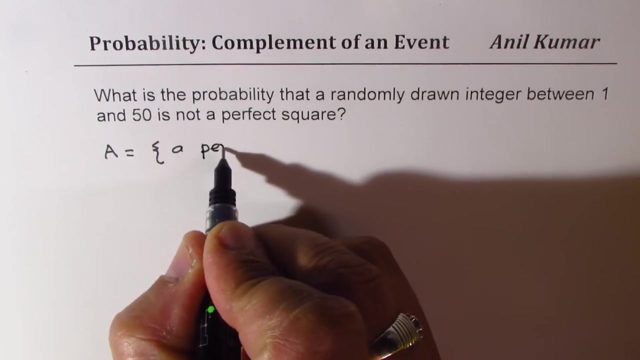 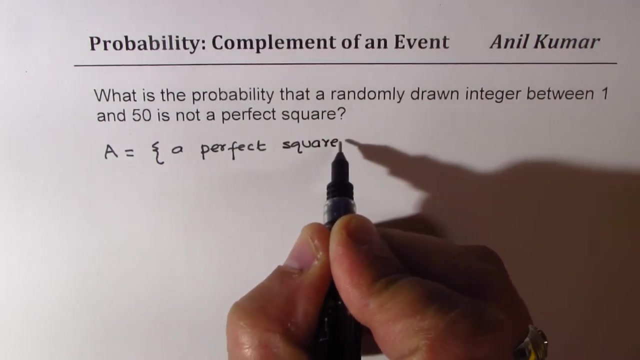 So, to begin with, we can define our event A as the one which is perfect squares, right? So event A could be defined as a perfect square. We know there are limited perfect squares, between 1 to 50.. When we say perfect squares, what numbers are we looking into? 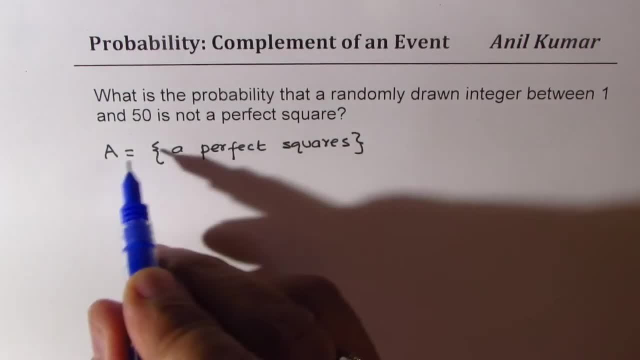 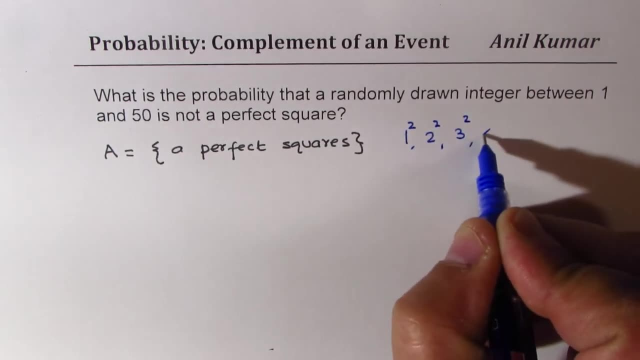 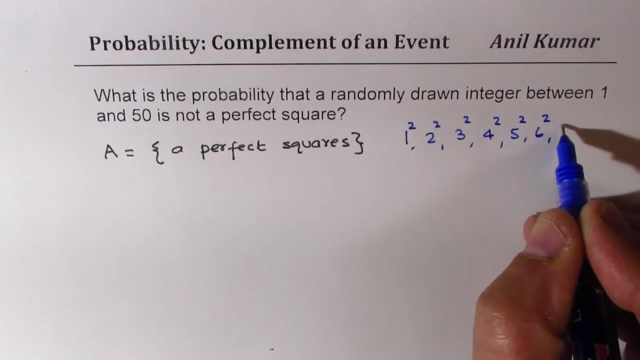 Well, for integers between 1 to 50,, it is 1 square which is 1.. 2 square is 4.. 3 square is 9.. 4 square is 16.. 5 square is 25.. 6 square is 36.. 7 square is 49, right, So these are the. 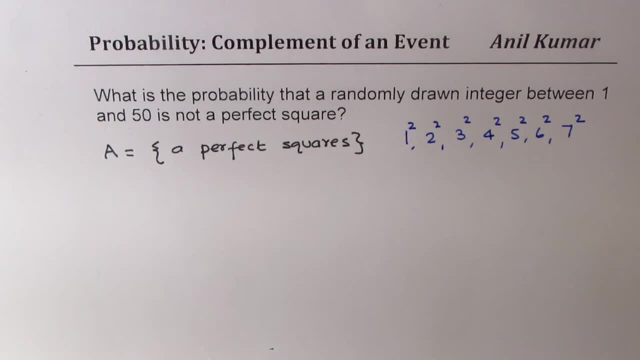 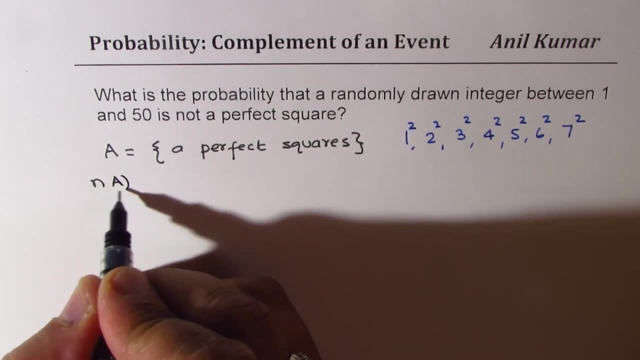 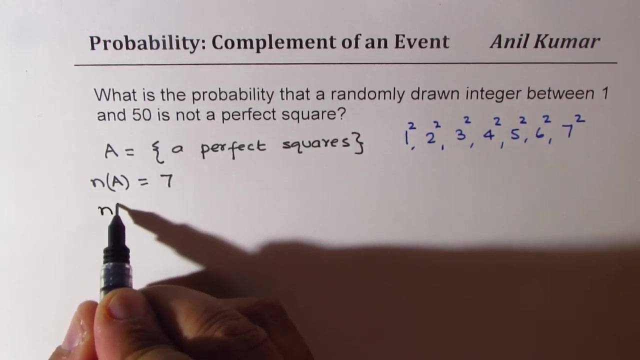 perfect squares, seven of them, which are total number of favourable events, right? So for us, N of A will be equal to 7, perfect. now in the sample space, what we have is 1 to 50, both included. we have 50 numbers, right. so the probability of picking up a? 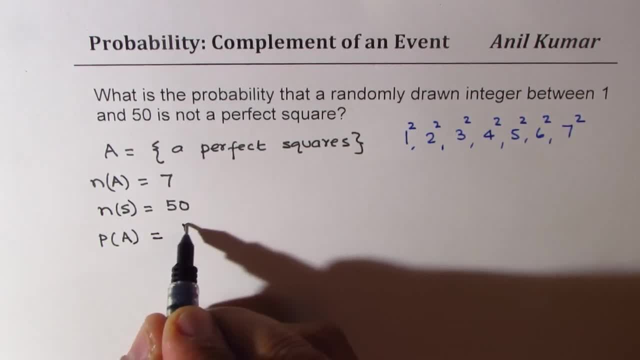 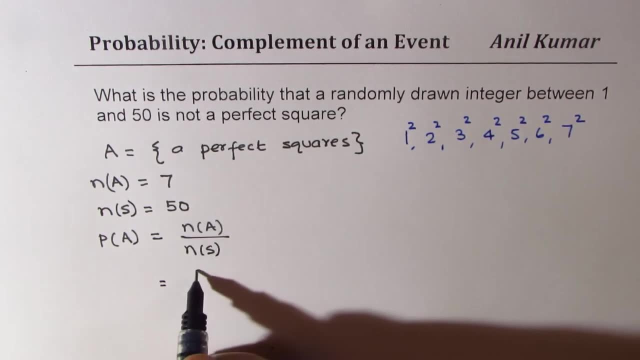 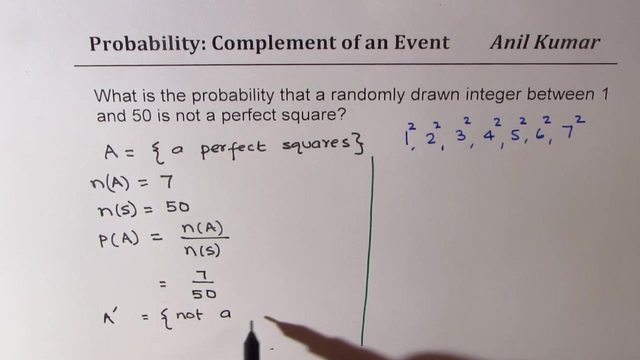 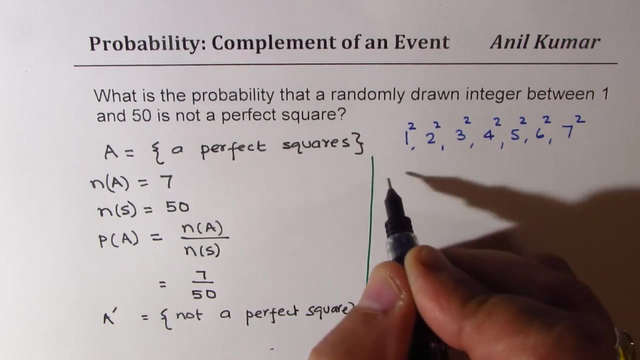 perfect square will be n of a divided by n of sample, so which is 7 over 50, correct? now we are really interested in finding that is not a perfect square, right? so? so the event which we are interested in is complement of a, which is not a perfect square. so to find the probability for the complementary, 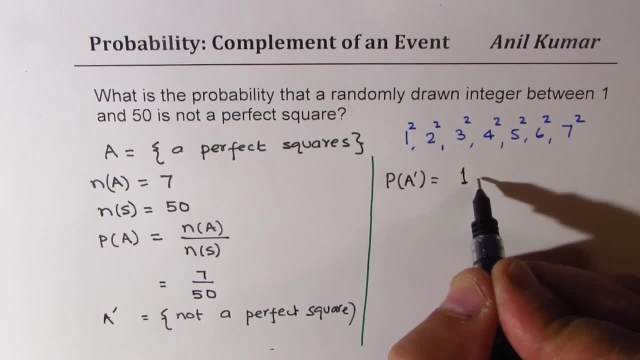 function. we know the sum of probability should be 1, so it is 1 minus P of a. so we could use this property and find the solution perfect. so we get 50 minus 7 over 50 as our answer, which is 43. perfect. so we get 50 minus 7 over 50 as our answer, which is 43. 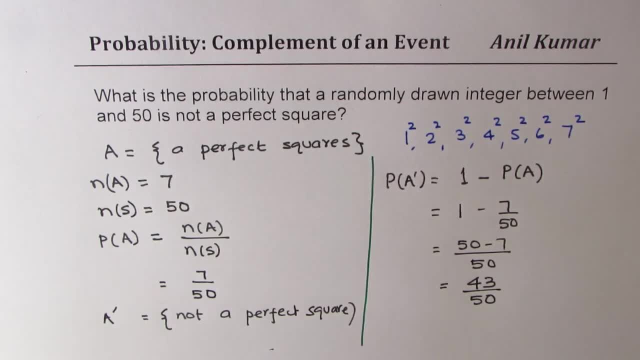 perfect. so we get 50 minus 7 over 50 as our answer, which is 43 over 50, correct. so in percent, if you want to change this, you have to multiply by 2 and say or so times 100 will be 86 percent. okay, so that is how.